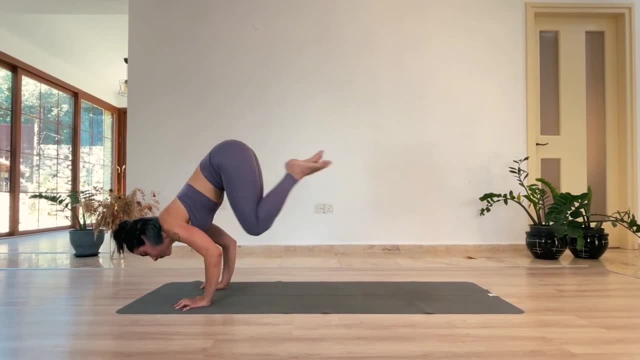 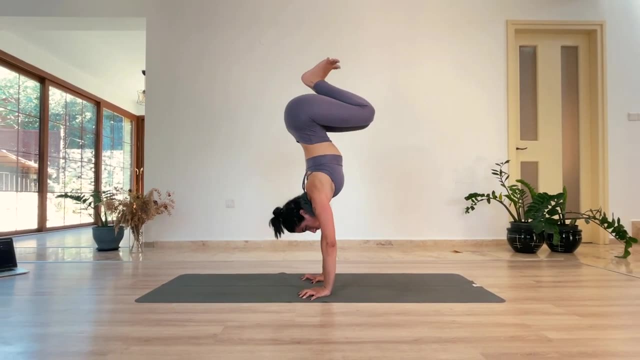 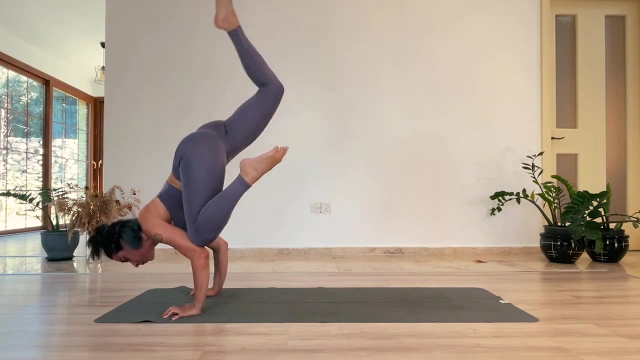 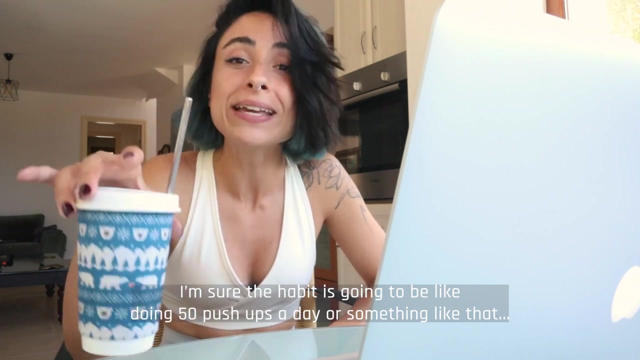 floating, jump backwards into plank, tuck handstand, crawl to handstand, transition or the combination of all of them. Okay, I'm sure the habit is going to be like doing 50 push-ups a day or something like that. The practical thing. 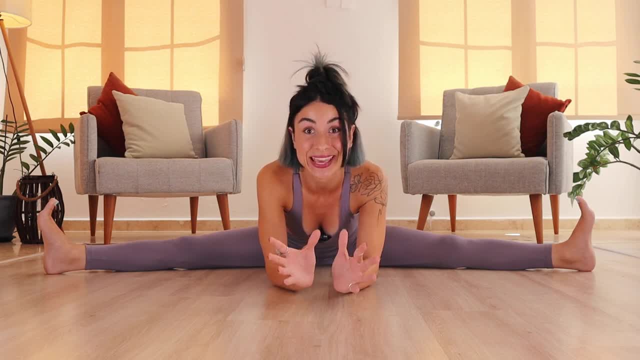 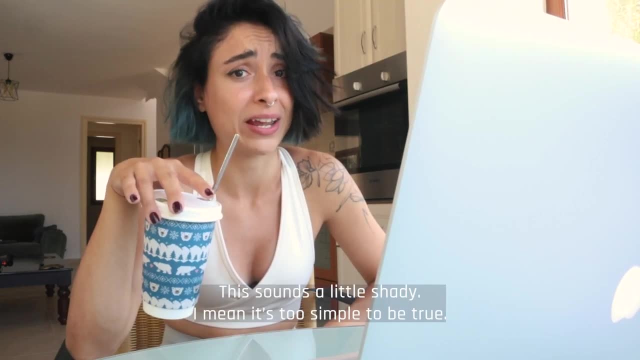 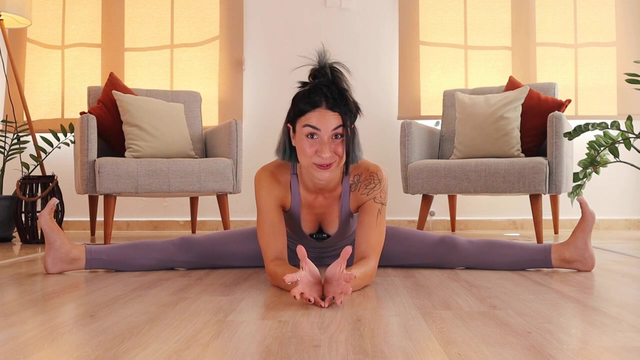 that will unlock all of these for you is actually pulling the knees to the chest. What? This sounds a little bit shady. I mean, it's too simple to be true. I know it sounds shady because it's too simple, but it is true. Let me show you what I mean. 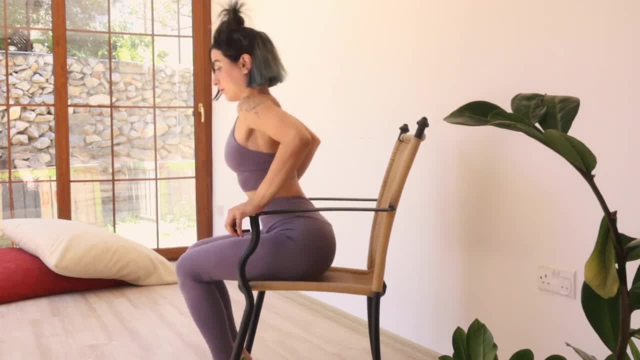 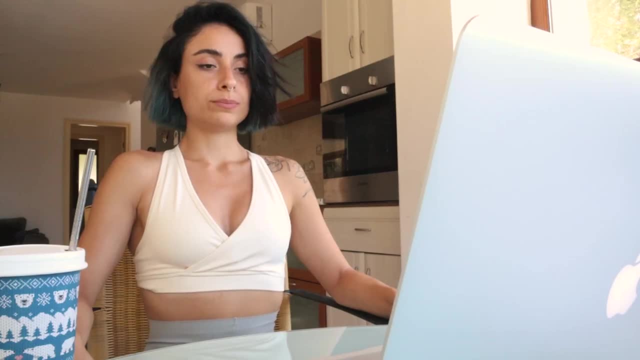 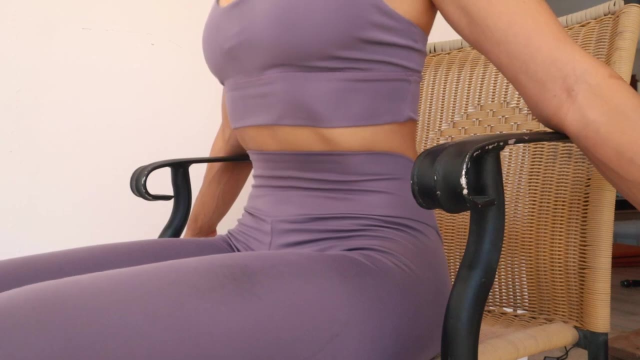 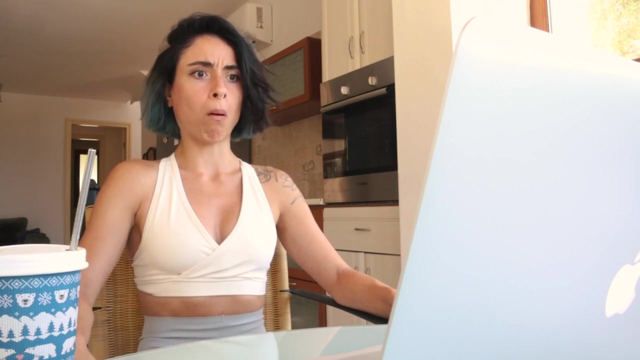 I am guessing you are sitting right now. If not, sit on a chair or something similar, Perfect. First inhale, Lengthen through the spine As you exhale slightly, throw up your lower belly and push your tailbone down. Even right now you might be feeling your lower abdominals. 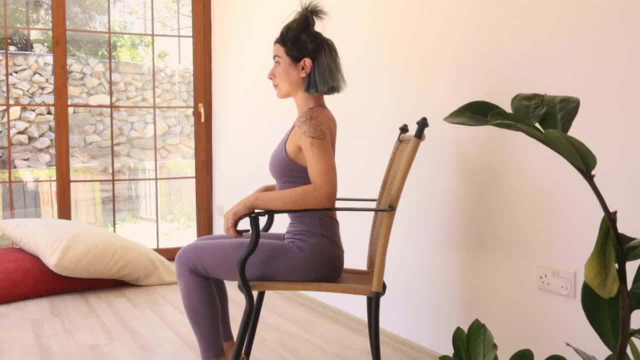 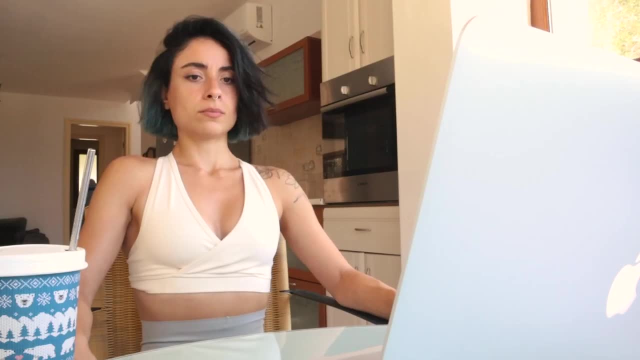 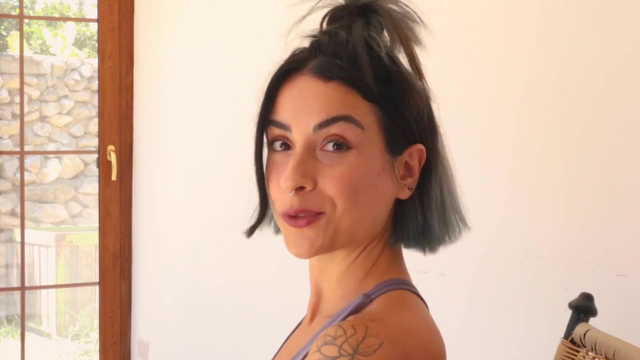 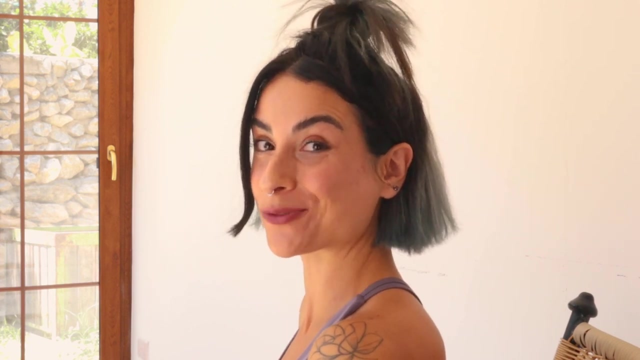 Now maintaining this posture. inhale first. As you exhale, start bringing one knee towards your chest, Close your eyes and hold it here. Do you feel it? Oh yes, This is how actually pulling the knees to the chest feels like. Put this sensation. 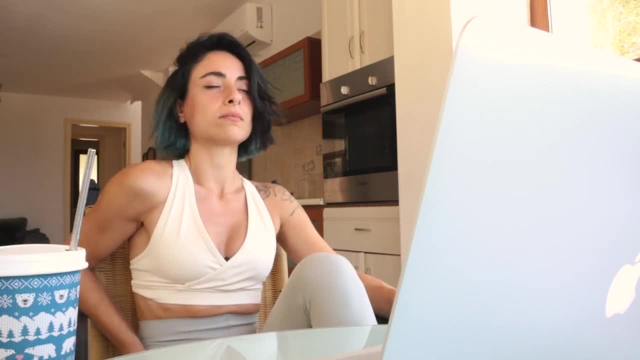 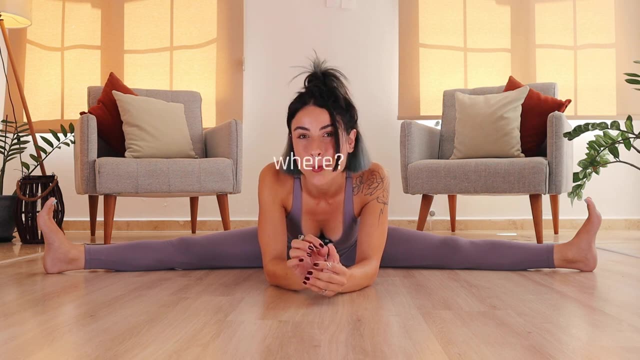 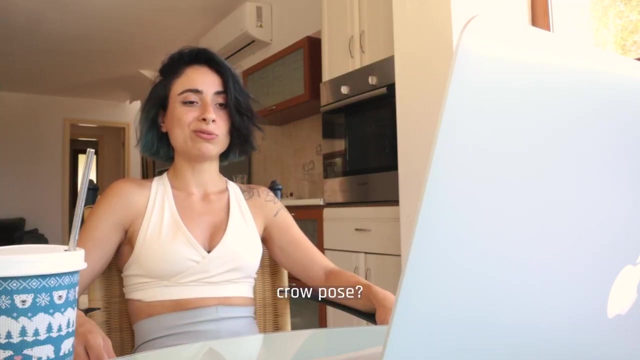 into your pocket. Save it So next time you're on the mat, you know what to look for. Now question: Where do we look for this sensation during our yoga practice? Crow pose- Accept the crow pose. How about bringing the foot forward? 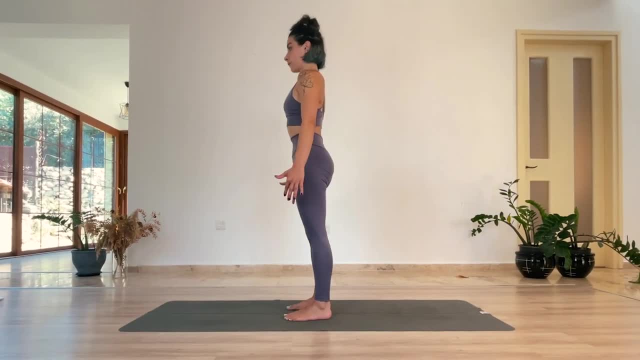 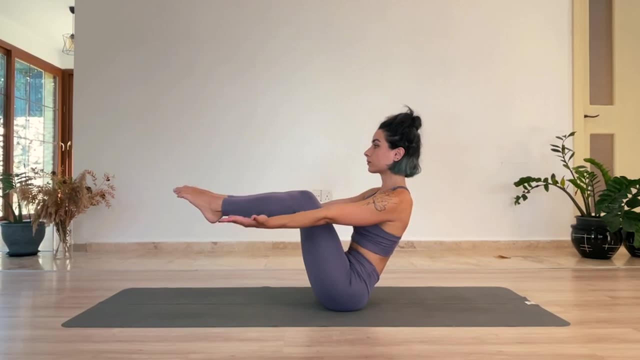 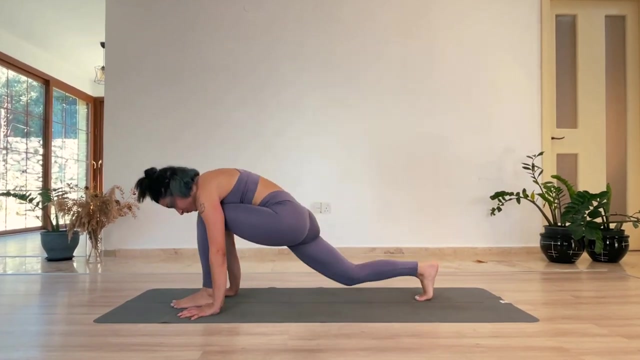 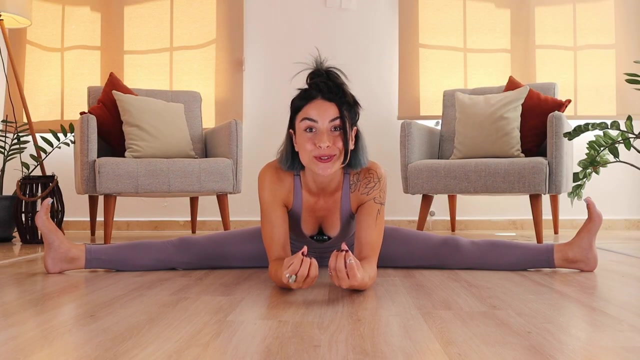 Half standing forward, fold Standing and pulling the knee to the chest, Chair pose, Bolt pose. If you teach yourself this element of compression in easier settings, like the ones that we mentioned, and turn it into a habit as you go through your journey, more complicated positions and